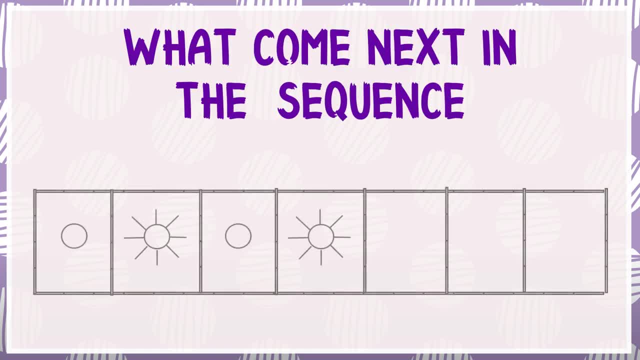 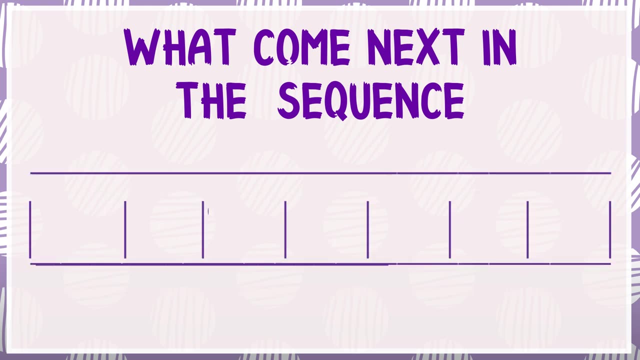 Square triangle, square square triangle. Square triangle, square square triangle, Square triangle, square square triangle. What comes next in the sequence? Circle sun, Circle sun. So what will be next? Circle sun Circle, Flower leave. 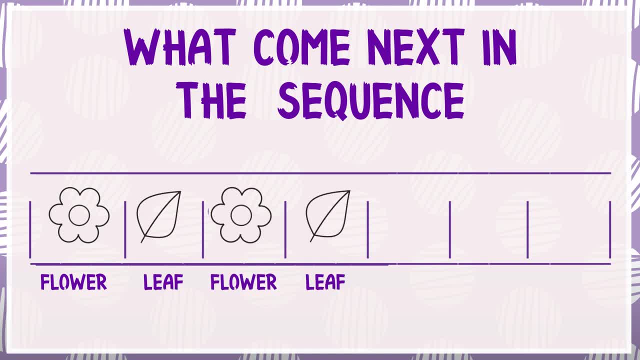 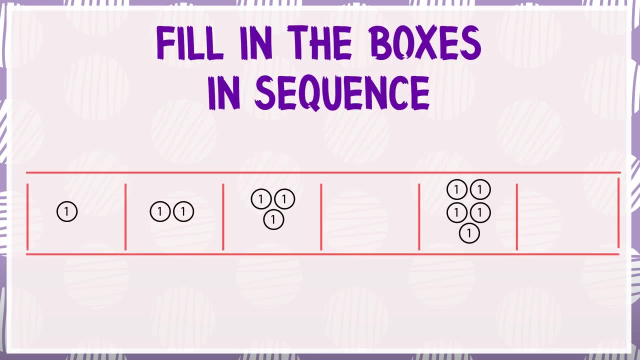 Flower leave. So what will be next? Flower leave, Flower. I have a last question, so please let me know in the comments below: Patterns in Shape: Fill in the boxes in sequence: one circle, one circle, two circles, two circles, three circles, three circles, and so will be. 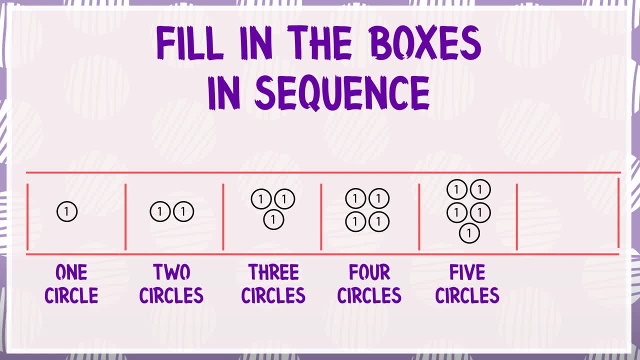 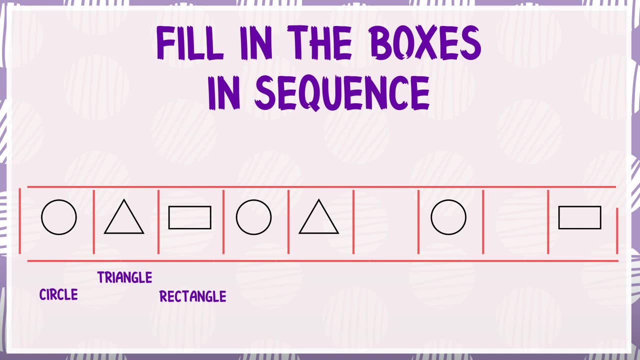 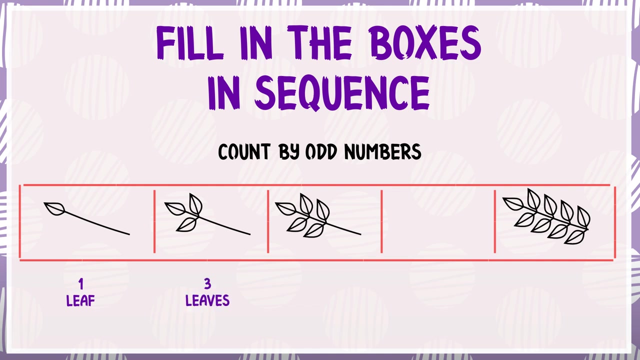 four circles, five circles, three circles, next circle, so next will be circles, circle level. and this circle Tri-amiento turned out, icons, simply turned out. concerns circle, triangle, rectangle, circle, triangle, so next is rectangle, circle, so next is triangle rectangle. one leaf, three leaves, five leaves, so next is seven leaves, nine leaves. 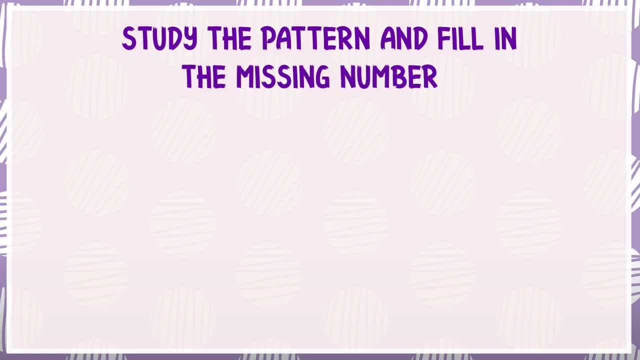 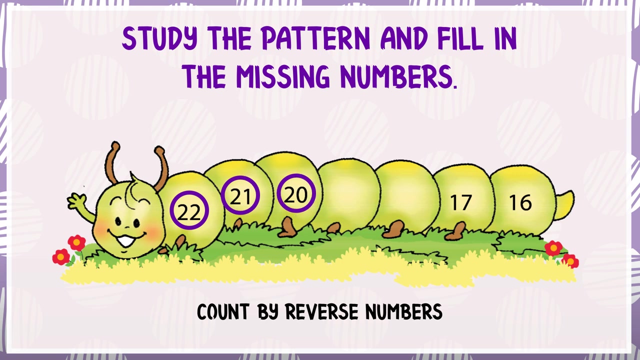 study the pattern and fill in the missing numbers: one, three, four, three, four, four, three, four, four, three, four, four, 5,, 7,. so what will be the next number? 9,. and after 9,, what will be the next number? 11,, 13,, 22,, 21,, 20,. so what will be the next missing number? 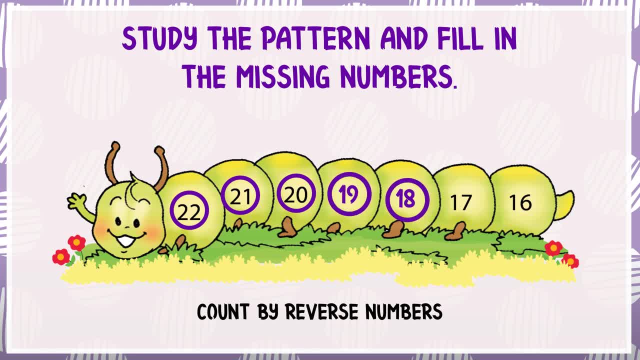 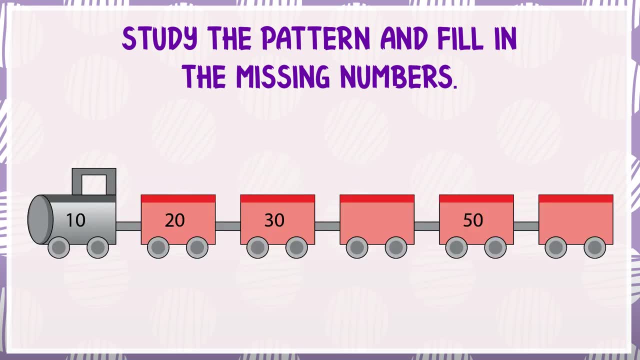 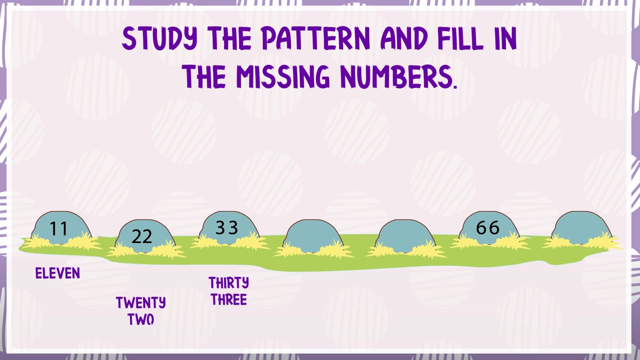 19,, 18,, 17,, 16.. 10,, 20,, 30,. so what will be the next missing number? 40,, 50,. what will be the next missing number? 60,, 11,, 22,, 33, so what will be the next number? 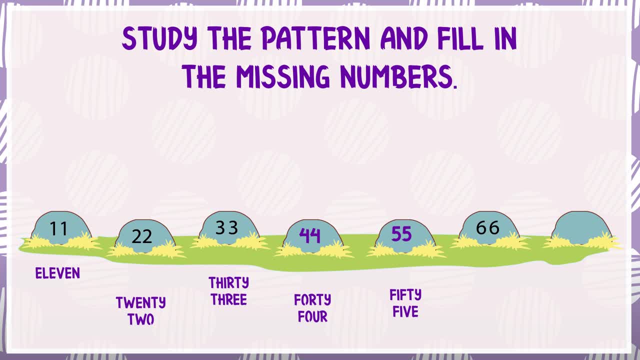 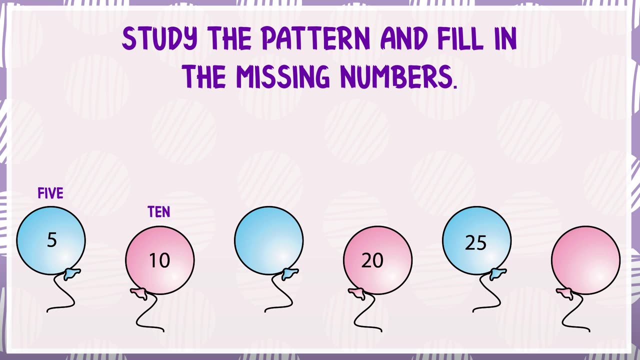 44.. 55,, 66,, 77.. 5, 10,. so what will be the next number? 15,, 20,, 25,. so what will be the next number? 30. 2, 5.. 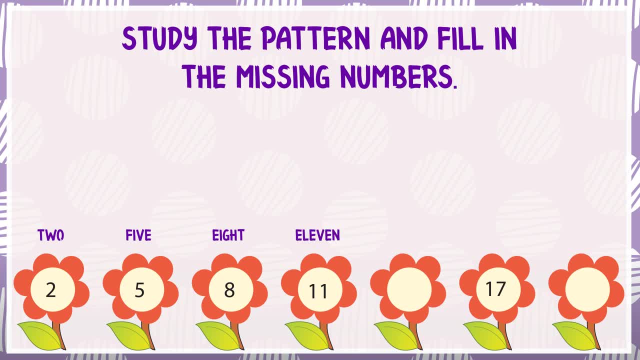 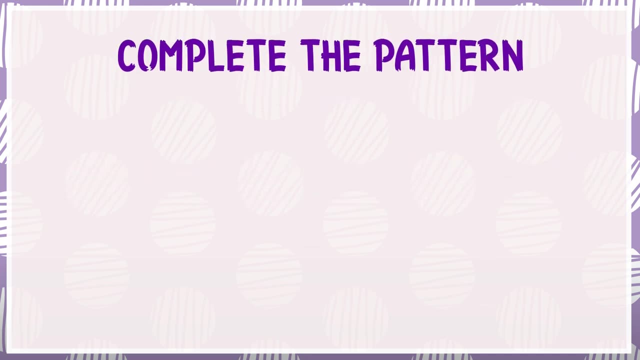 5,, 8,, 11,. so what will be the next number? 14,, 17,. so what will be the next missing number? 20. 20. Complete the pattern: 2,, 4,, 6,, 8,. so what will be the next missing number? 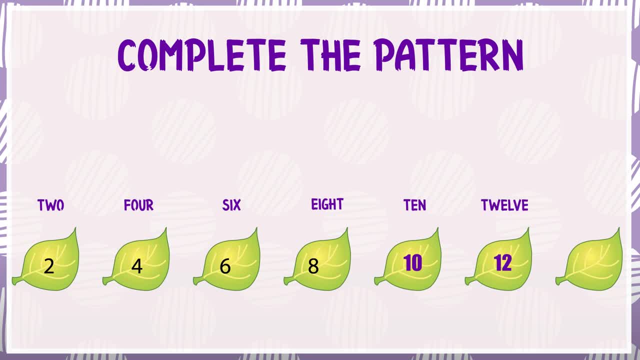 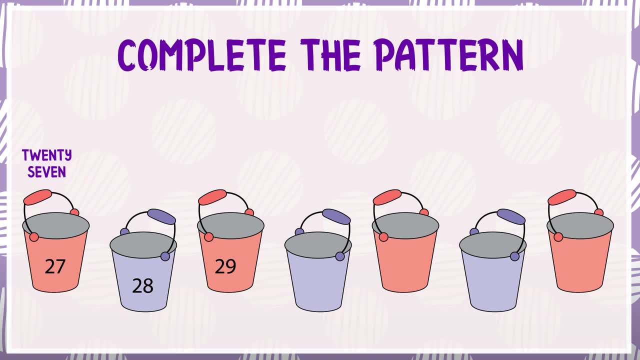 10. 12. 12. 10,, 11,, 12,, 13,, 14,, 15,, 16,, 17,, 18,, 19,, 20,, 21,, 22,, 23,, 24,, 25,, 26,, 27,, 28,, 29,. so what will be the next missing number? 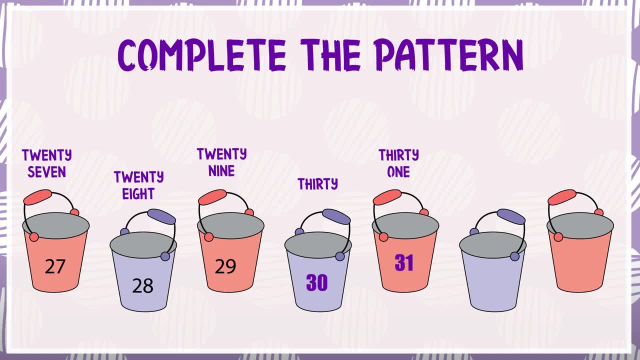 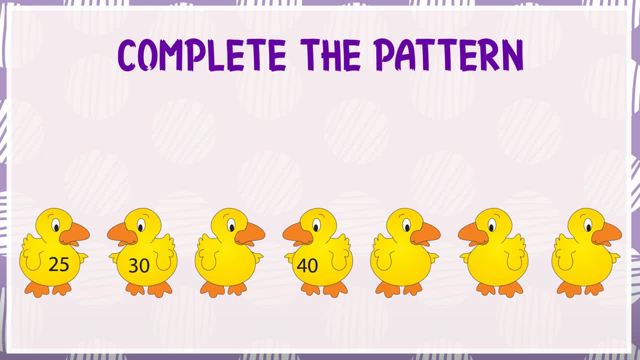 30,, 31,, 32,, 33,, 25,, 30,. so what will be the next missing number? 30,, 32,, 33,, 33,, 34,, 35,, 40,, 45,, 40,, 45,, 50,, 55. 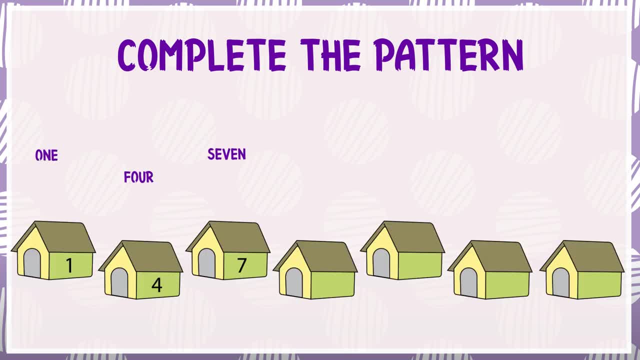 1,, 4,, 7, so what will be the next missing number? 10, 13,, 16,, 19.. 30,, 32,, 33,, 34,, 35,, 40,, 50,, 54,, 55.. 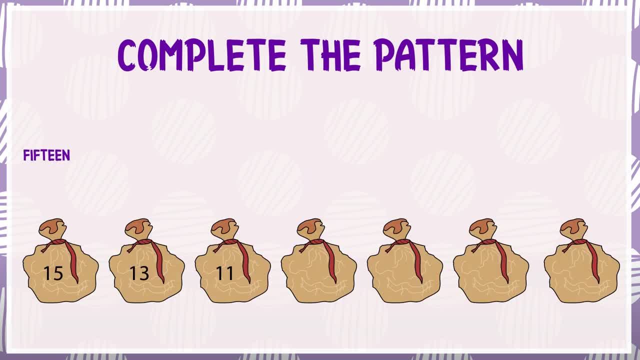 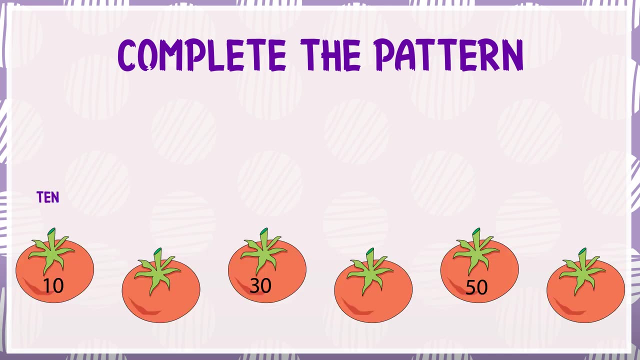 1,, 4,, 7, so what will be the next missing number? 10,, 13,, 16,, 19., 11. so what will be the next missing number? 9, 7, 5, 3, 10. so what will be the?